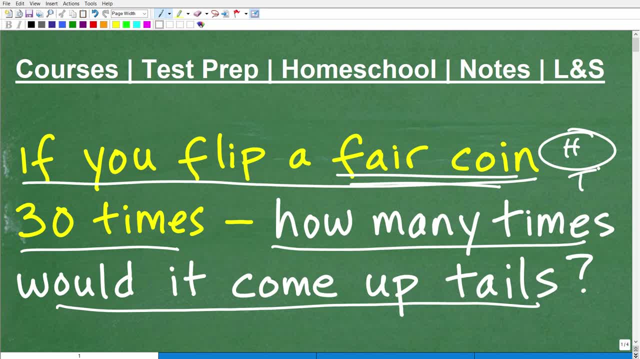 I absolutely love teaching mathematics. It is my true calling, And I can tell you right now all of you could be successful in math, And I'm especially speaking to those of you that struggle in math. Maybe your confidence in your ability to learn math is very low. I'm telling you right now you could do much, much better As long as you're willing to work hard. you have someone encouraging you to do well, all right to like, hey, keep going. We all need those people in our lives that encourage us, you know. so that's important. 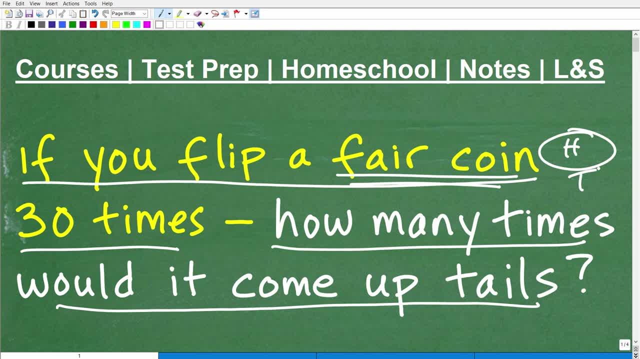 You know it could be your teacher, it could be a parent, it could be a friend, but hopefully you have some positive people uplifting you in your life. But the most important thing you need to learn mathematics is great math instruction- clear, understandable and comprehensive. 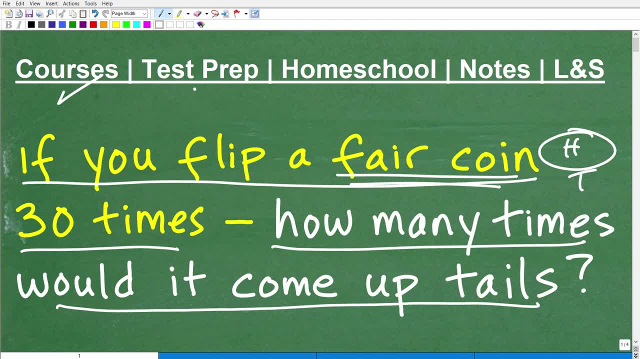 So, if you need help in your current math course or maybe some sort of special test that you're preparing for, something like, let's say, the SAT, ACT, ASVAB, GRE, GMAT, GED, a teacher certification exam, something that's going to have a major math section on it, 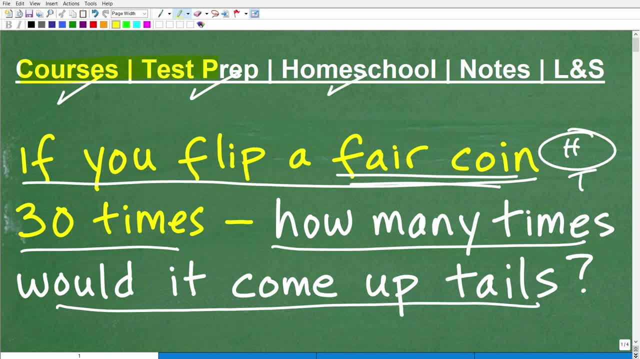 Or if you are homeschooling mathematics, check out my math help program. I'm going to leave a link to it in the description of this video. I literally have over 100 plus different math courses that span all these categories and much, much more. I'm also going to leave links to my math notes in the description as well, Because unfortunately, a lot of students don't take adequate math notes. Some students don't take any math notes. When I was taking notes way back in the good old days, back in the 1980s, when I was in high school, I would just like to take a math note. 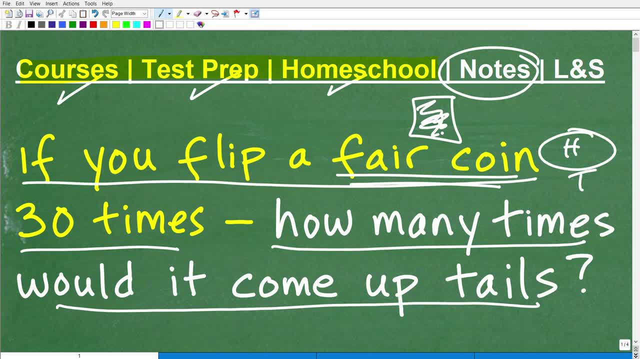 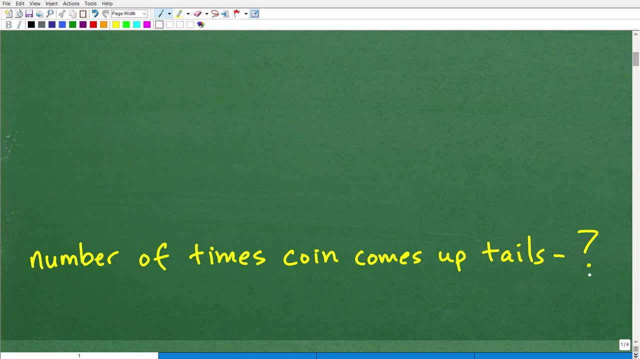 tails. well, the answer is: i don't know. okay, the number of times it comes up, tails is. well, that could. that all depends, right? uh, there is no answer, there is no precise answer, and just think about it. uh, you know, some of you might be saying, hey, this is a trick question. well, no, 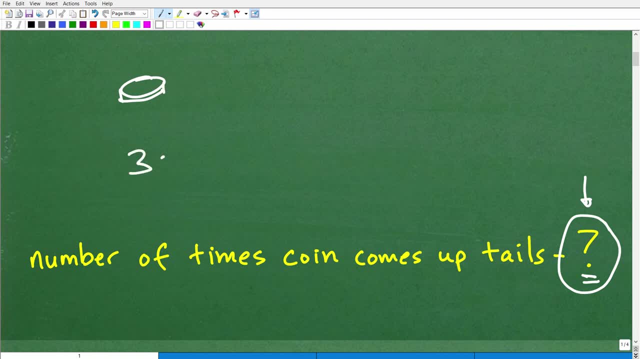 listen, if we had our little coin here, all right, and we flipped this thing 30 times, you know, kind of flipped it around and kind of spun up in the air or whatnot, it landed on the ground. you know, let's say you did this experiment, uh, uh, five times right, and uh, you know now most of you- 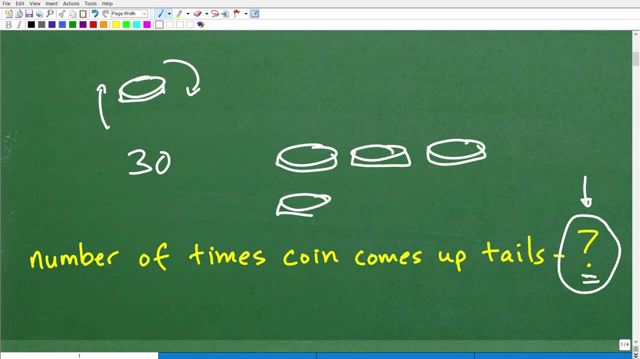 might be. so let's do it six times, all right. there's one, two, three. i'm kind of drawing my little coins here now. well, let's just kind of use some common sense, right? so here's heads and here's tails. now, how many times can, or what's the chances of the odds of this thing coming up? tails: 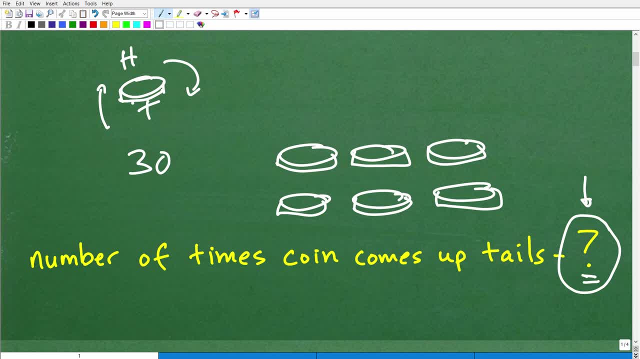 well, most of us just like: don't you have a one out of two chance of coming up tails? yes, that's absolutely right. but let's suppose you just flip this coin, uh, six times, right, let's think of some possible outcomes. uh, maybe it would come up tails, all right, maybe. 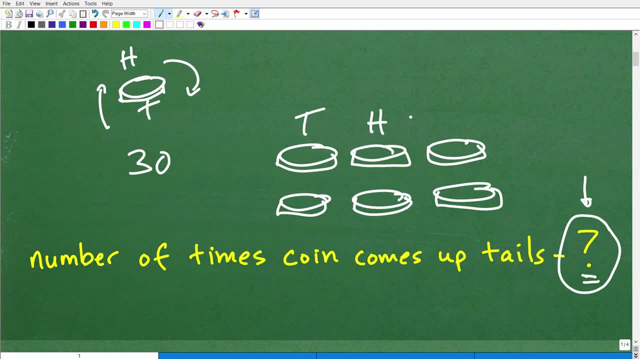 you know it's not going to come up like say, oh, tails, and then it comes up heads again. oh, it comes up tails and it comes up heads. and it comes up like that's alternating. just because it has a one out of two chance, all sorts of crazy stuff can happen. right, you could flip this uh coin, uh. 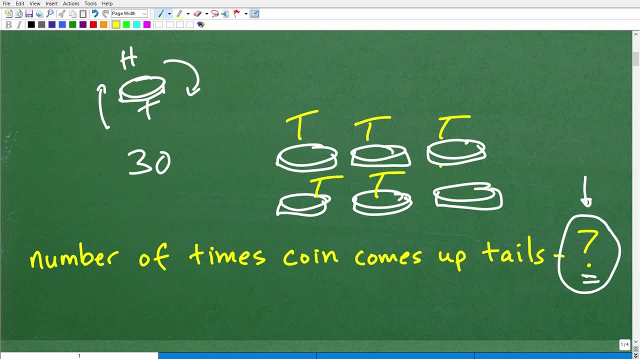 six times it could come up tails, and then it comes up tails, and then it comes up tails, and then it comes up tails, tails, tails, tails, tails, and then maybe it hits right. it just you just don't know, we can't predict this. so you know, there is no definitive, absolute way we can predict the future. 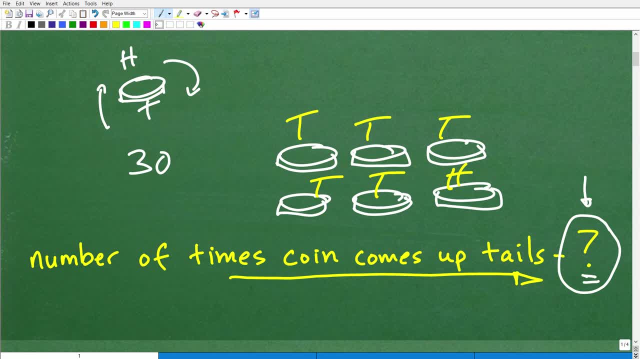 if you do know an absolute way to predict the future, definitely let me know, because you know that would be pretty, uh, a pretty valuable skill, right? so we're talking about probability. what's the chances of something happening? well, that's different. okay, we can get a sense of, uh, the 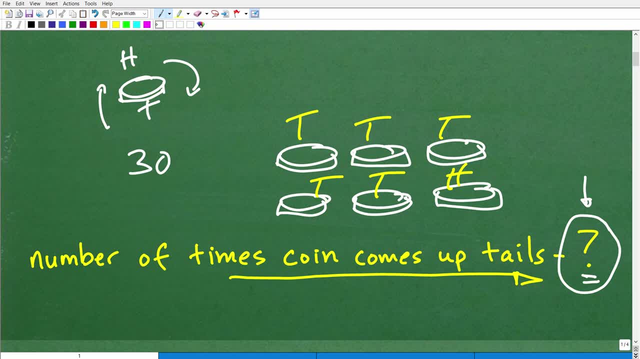 chance of something that might occur. now, if you said the number of times you can come up tail is 15 times, well, that is a reasonable guess, right? 15 out of 30 times it would come up tail. that's a reasonable guess, but there's absolutely no way that we can guarantee that. we know exactly that. 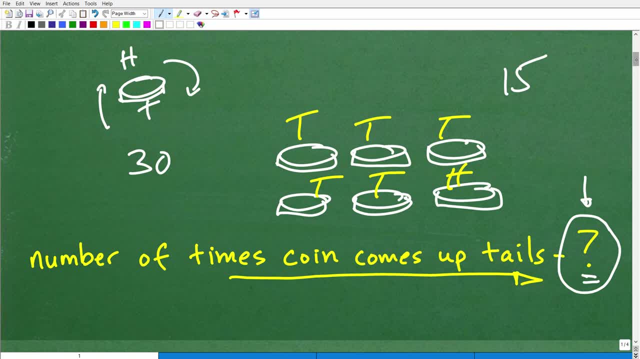 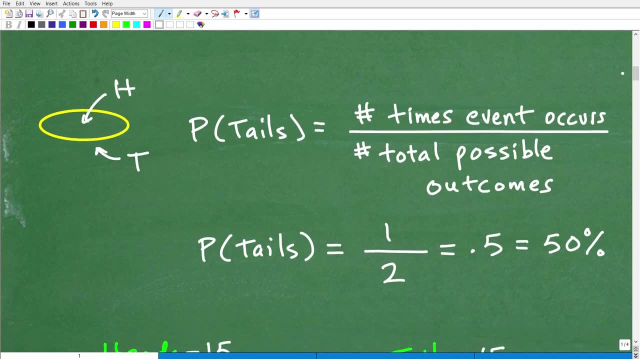 in fact that is going to be the case, but let's talk about some really big picture, basic concepts and probability. that is really going to then kind of tie in all these concepts i'm talking about. all right, so first of all we want to define, um, the basic, uh, definition of a probability of an. 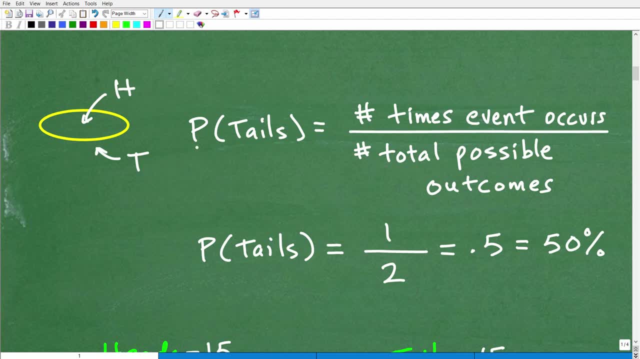 event. okay, so here is our fair coin, here's heads, here's tails. so the probability of um, this coin coming up tails right. this is the, uh, what we call the theoretical probability. well, that's going to be equal to the number of times this event can occur over the total possible outcomes of events. 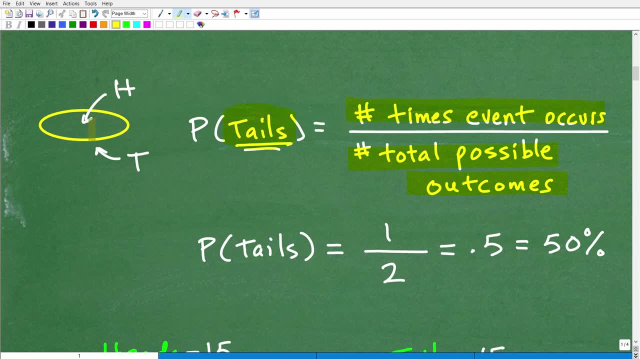 well, what does that mean? well, how many ways can this coin come up tails? right, there's only one way this coin could come up tails, and that is if it lands and we see the tails right. so there's one uh way this coin could come up tails. 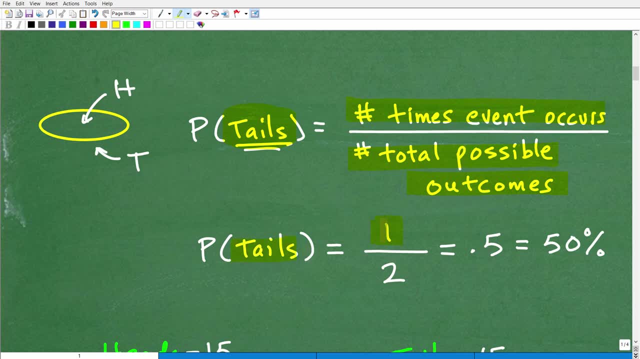 but what's the total possible outcomes? well, it could come up two different ways: heads or tails. that's a total possible way, so it could come out one out of. we have one out of two, um possibilities of this thing coming up- tails. so we have one over two. 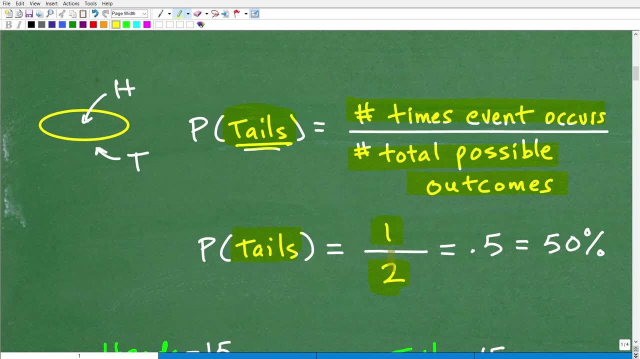 and a probability. we like to express the probability in terms of percent. so one half is the same thing as 0.5 or 50. we have a 50 expected um probability that this fair coin will come up tails. now, that's what we expect from a theoretical standpoint. okay, but again. 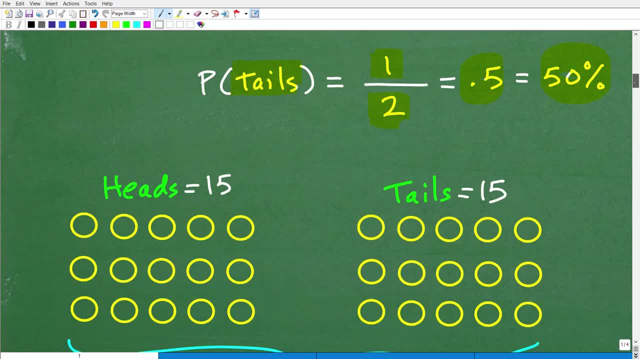 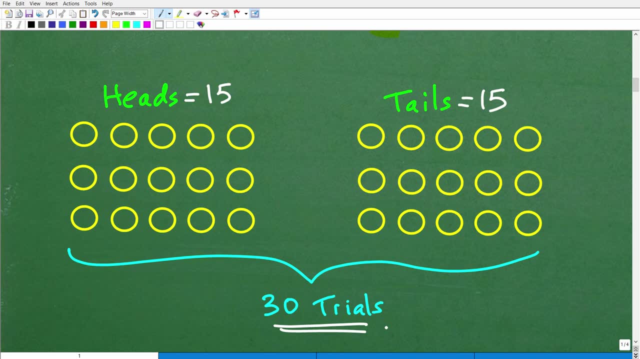 is there any guarantees? well, no, okay. so let's kind of take a look at the theoretical standpoint, at this theoretical probability. so here is 30 trials, let's get our coin out and let's flip this thing. so this is not the way the real world, uh, works right like, okay, you know, um, yeah, 50 of. 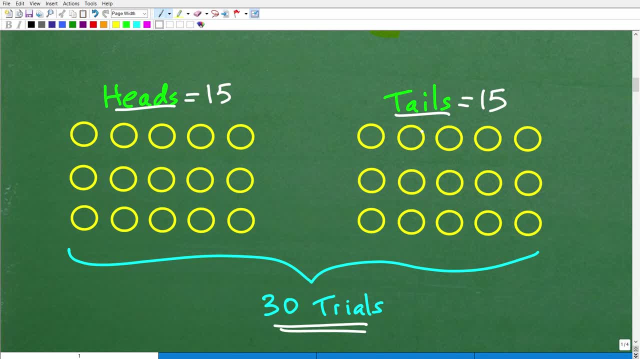 the time that this coin is going to come up- tails. so i flipped this thing 30 times: uh, here we have 15 uh results that are heads, and then here are 15 times the results were tails. is this the way real life works? no, it does not work this way. 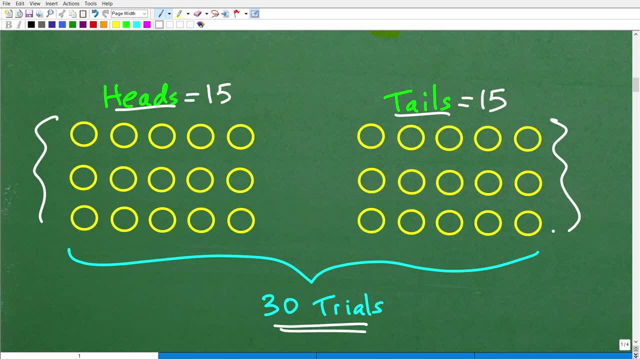 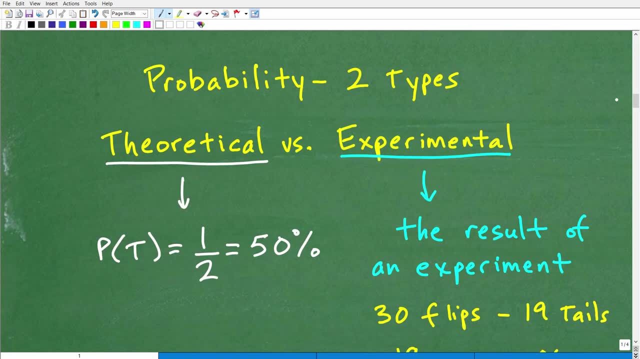 okay. so here's the deal. when we're talking about probability, there's basically two types. okay, there's two types of kind of real, uh probability. um, that's kind of going on here right. there are two big picture concepts about probability. the first is theoretical probability, and that's what. 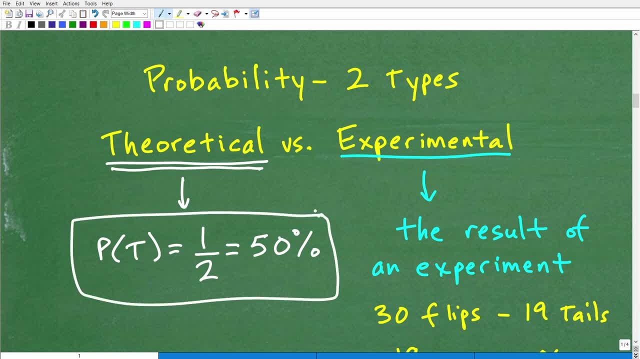 we're doing um with this definition of probability. we're just trying to get like: what is the expected outcome of this event occurring? so again, the probability of this fair coin being a tail. we have a one out of two. uh, two outcomes, right. so that's 50. that's theoretical we would expect. 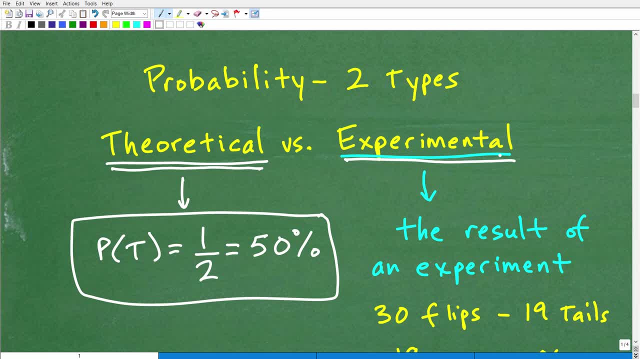 15. but we have this other probability and that's called experimental. let's suppose we're like: well, what's the let's? let's go ahead and put this to the test. so here, what we could do is run an experiment. okay, so we're going to put this to the test, and we're going to put this to the test, and 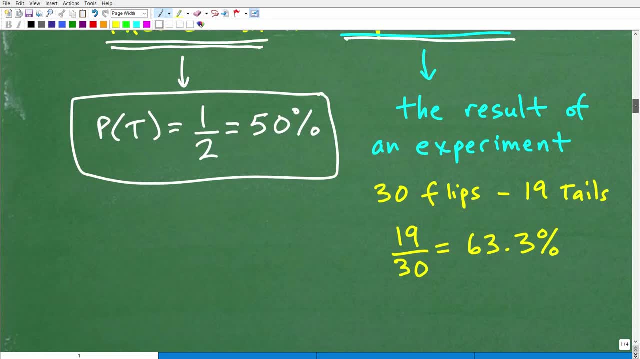 okay, so let's suppose we run this uh experiment and we're going to flip this coin, uh, 30 times. we do 30 flips. we're like and let's, let's going to take this 50 probability expectation and let's put it to the test. well, we do 30 flips and guess what ends up happening? we get 19 of um those flips. 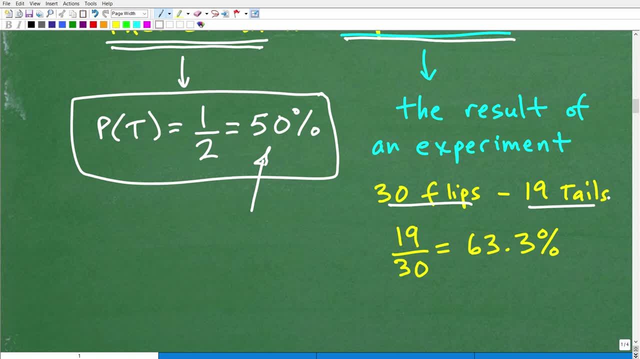 come out to be tails. so let's go and count, uh calculate the actual percentage, the chances of this coin flip coming out to be tails. we're going to put that's going to be 19 out of 30 times, so 63.3 percent. okay, so interesting. so we have a fair coin. are we saying that every time you flip? 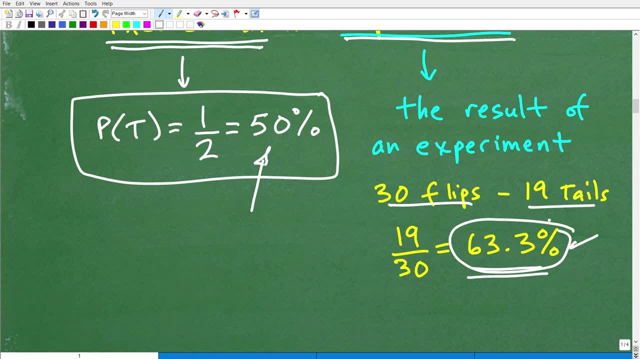 a fair coin, you have a 63.3 percent of it becoming, you know, landing on tails. well, that doesn't make sense, right? because we would expect that we um only really have a one-half chance, right? uh, 50 chance of it becoming, uh, tails. so what's the deal here? we run this experiment. it's like 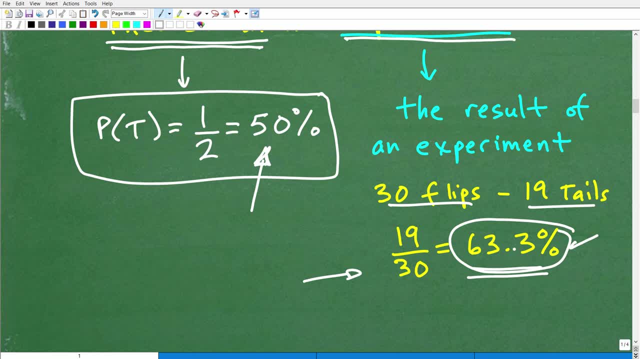 well, it looks like we get tails, uh, more frequently than you know hits. okay, you know how can we resolve that with our expected probability of 50 of the times we get tails right. so we have like something we have to resolve here. well, what we need to resolve is the following: okay, you need to. 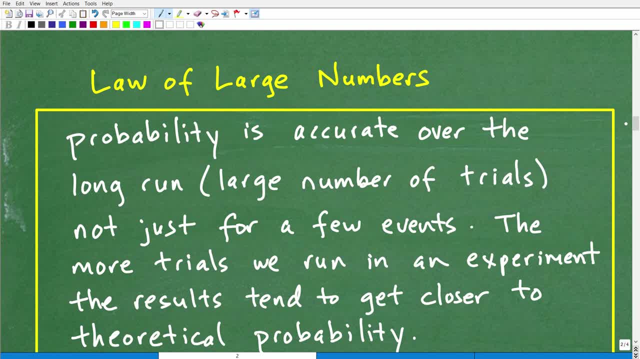 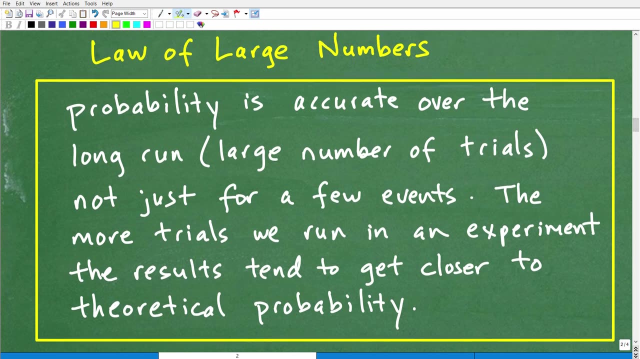 have an understanding of this thing right here, and this is called the law of large numbers. all right, if you never heard of this, this is very, very important, extremely important, and i'm going to go ahead and read this to you and then, basically, this is going to kind of wrap up this video. let's go ahead and read this here. 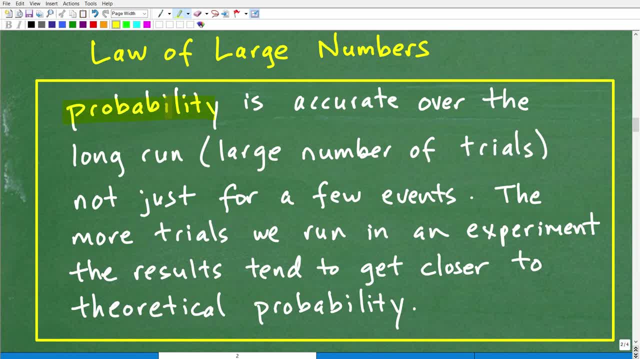 so it says the probability. and, by the way, there's a lot of different ways you can express the law of large numbers. if you're in a more advanced probability class, it's a little more technical way you can express this, but i'm going to use this language here. probability is: 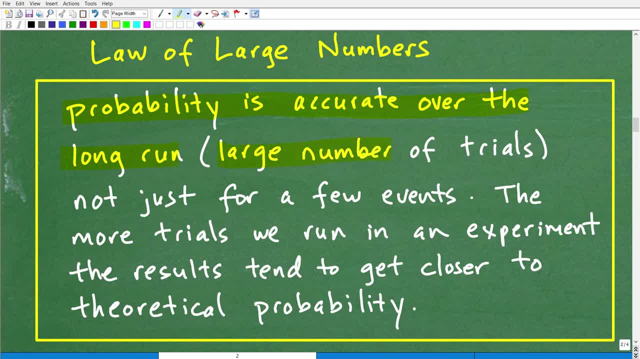 accurate over the long run. okay, the larger number of trials, not just for a few events. okay, what we're talking about here is this: um, if you- just, you know, run a few experiments, like if we flip our coin a couple few times, uh, six times, and, like you know, five out of six times it comes. 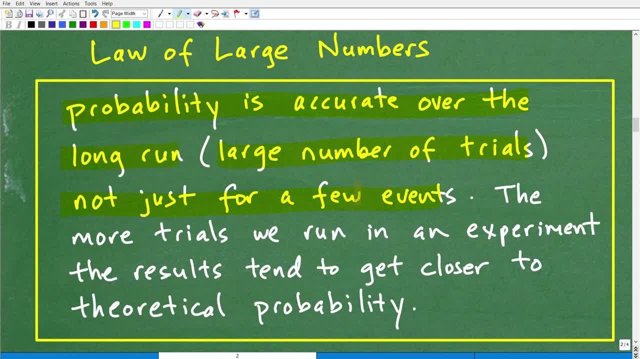 up tails. that's not really good in terms of its accuracy, or uh. so here's the deal: the more trials where you run in an experiment, the results tend to get closer to the actual number of trials and closer to theoretical probability. this is the key concept. you need to know the law of large numbers. 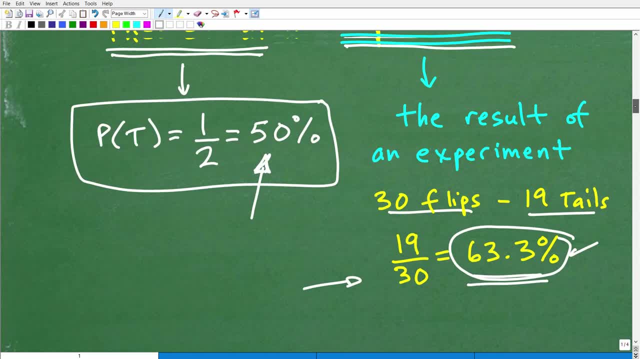 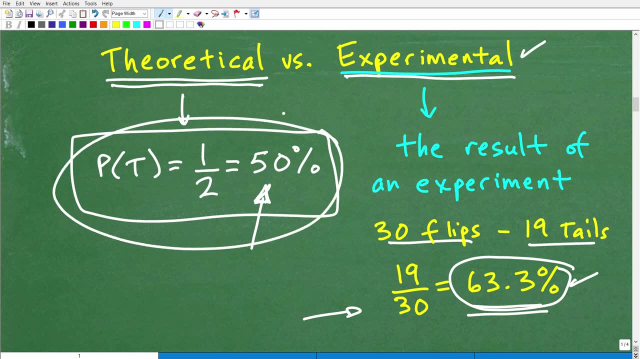 so let's go back to this little deal right here, this experiment. okay, so we have this theoretical probability that a 50 of the time we are going to get, um, tails. well, we do an experiment for 30 flips and we only got tails, uh, 63.3 percent of it, or we got tails 63.3. 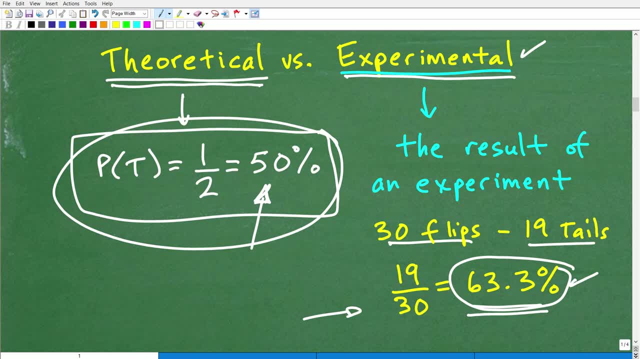 uh, percent of the time. well, guess what if we increase more trials or we add more trials to our experiment? so, instead of 30 flips, let's go ahead and do 300 flips as an experiment. how about 3 000? okay, how about you know, we do you know? 3 billion, it doesn't make a difference, the larger. 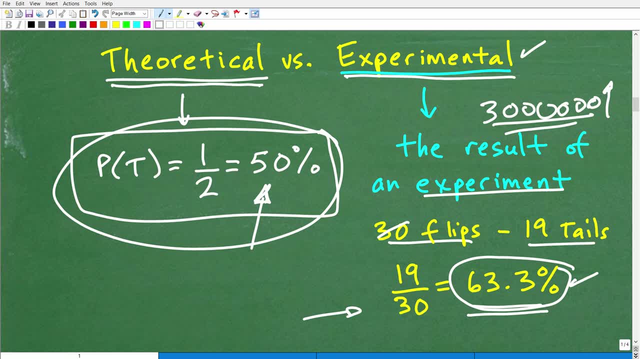 this number goes up. okay, the more trials we run, guess what's going to happen to our results, this result here. it's going to get closer and closer to the actual number of trials that we run- 50 percent. so if you take a fair coin and you flip it three trillion times, you can pretty much 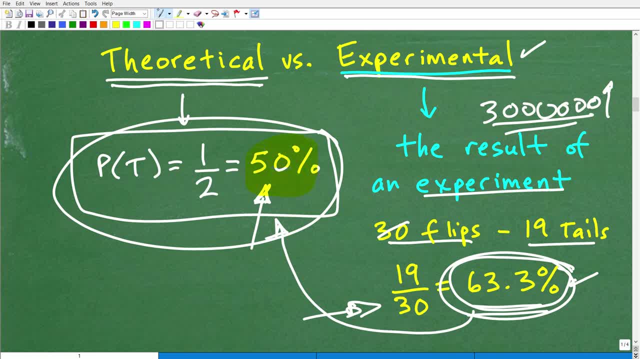 rest assured that almost, uh, precisely 50 percent of the time you will get tails and 50 percent of the time you're going to get heads. it's going to be like a promise: 50, 50 match right. so that is the uh, an illustration of the law of large numbers. so just because you have a theoretical 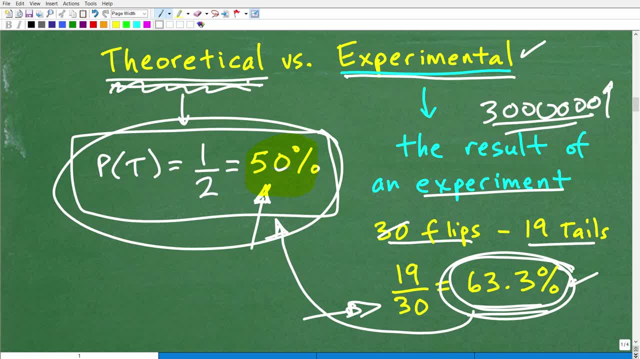 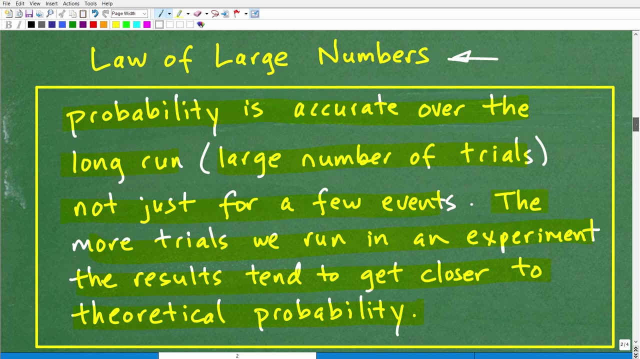 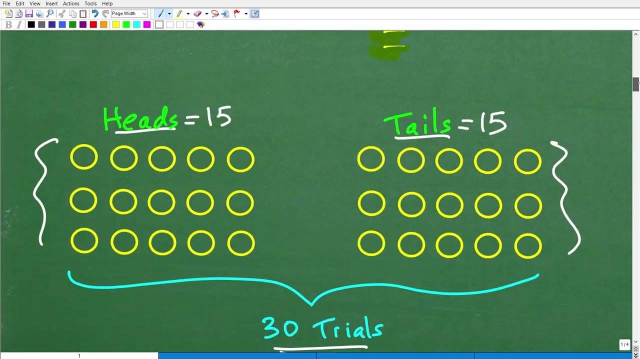 calculation of the number of trials that you're going to get tails and 50 percent of the time you're still having twoOUT the probability of that it's scored as a much larger probability. year of our probability is what we're trying to predict: outcomes right, it's a predictive thing, so 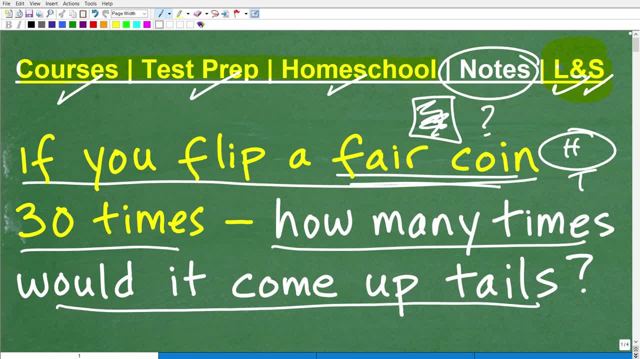 what's the chances of something, What's the chances of you know? you know what the weather. you know it raining tomorrow. what's the chances of whatever the case is right? We hear this all the time In our news. we're talking about, hey, the chances of win the lottery, the chances of it. 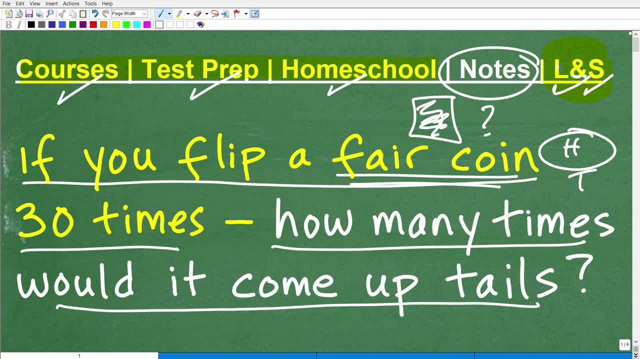 raining what's the probability or what's the chances of this person winning the election. whatever the case is, the better you have a better understanding of basic probability concepts like the law of large numbers, the better off. you're going to be All right. so if you need help with 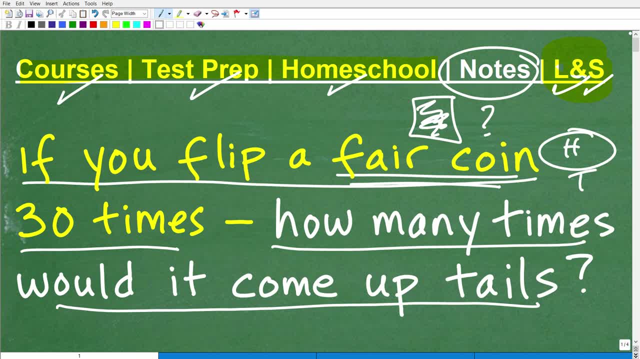 some basic statistical concepts like this. I teach this stuff in like part of my algebra courses at various levels So you know you can check out, like my pre-algebra course and my algebra course. I do have a chapter on data and basic statistics and data and stuff like that, So kind of get into.